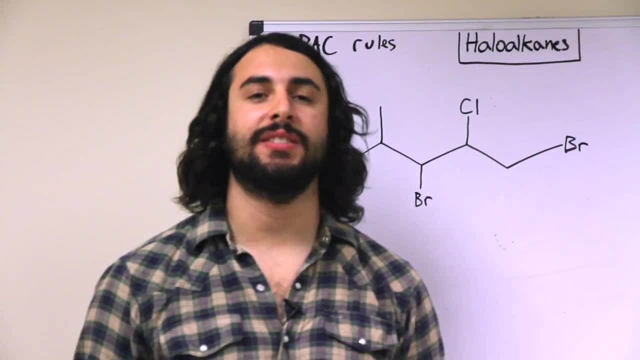 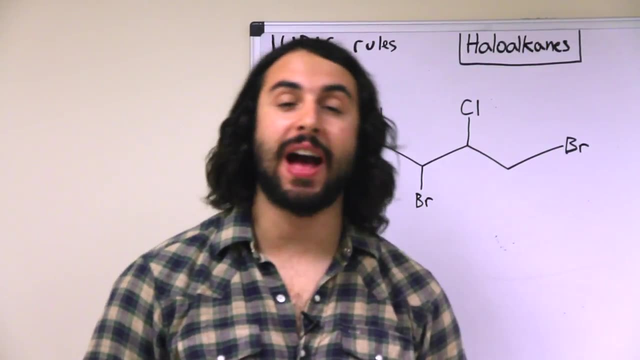 now let's take a look at some other kinds of substituents other than alkyl substituents. very common one is halogens. when you have a hydrocarbon with halogen substituents, these are called haloalkanes. so here's one now. all the 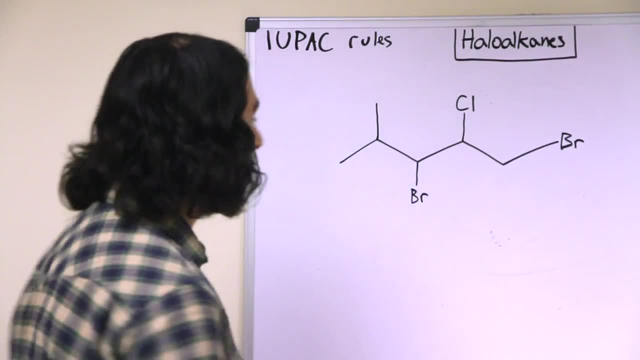 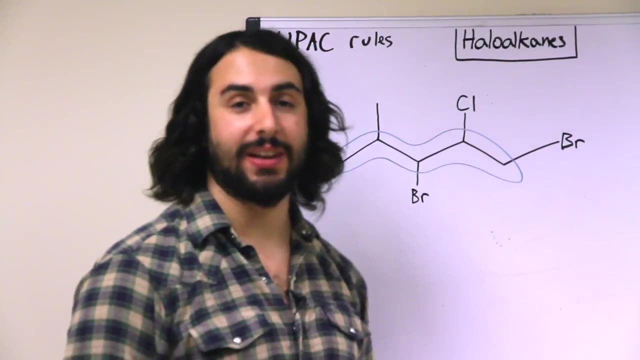 rules are the same. so first we're going to identify the longest carbon chain, being very careful to realize that this bromine atom is not a carbon atom. right, this is a bond to a bromine atom, so that does not count as a carbon. so we have a. 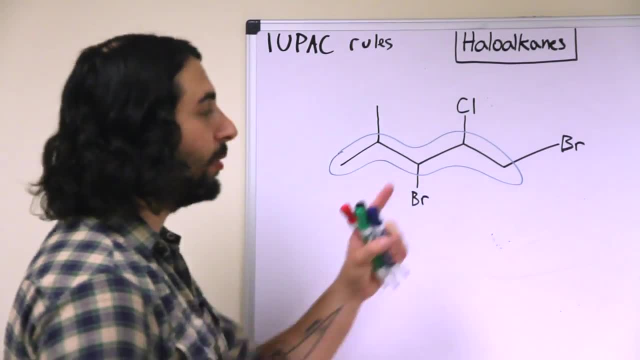 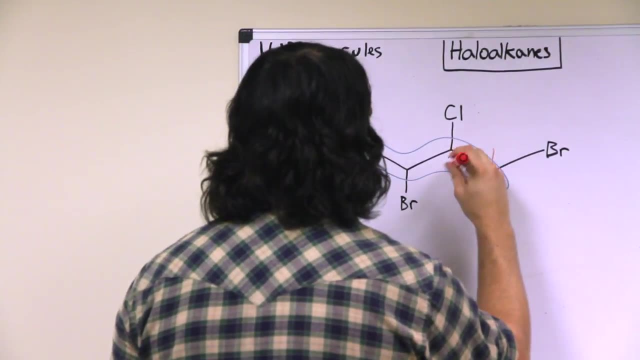 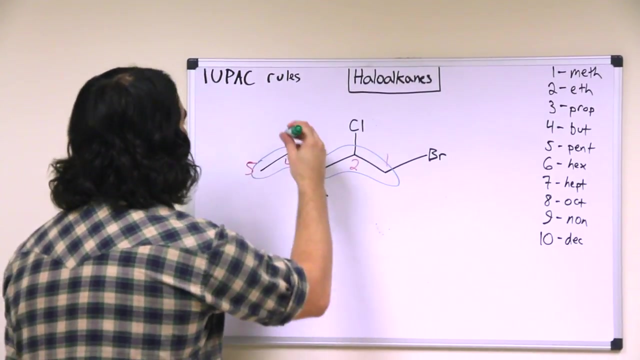 5-carbon chain. now we are going to number right to left, because there is a substituent on carbon 1 on this side now. luckily, the rest is the same at this point. so we're going to see that we have a methyl group and then we have three. 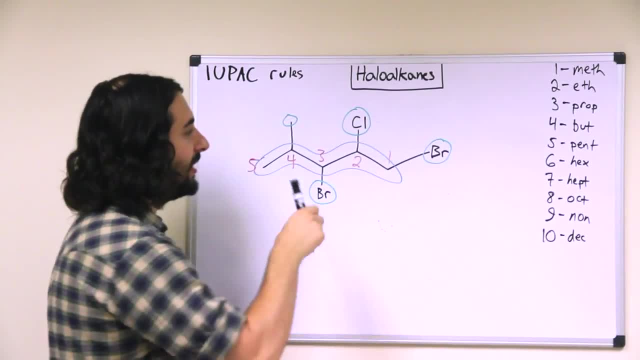 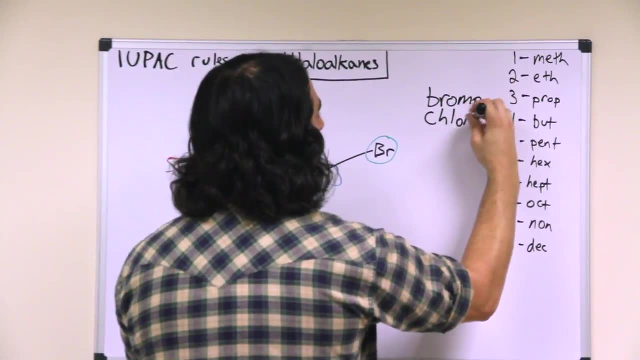 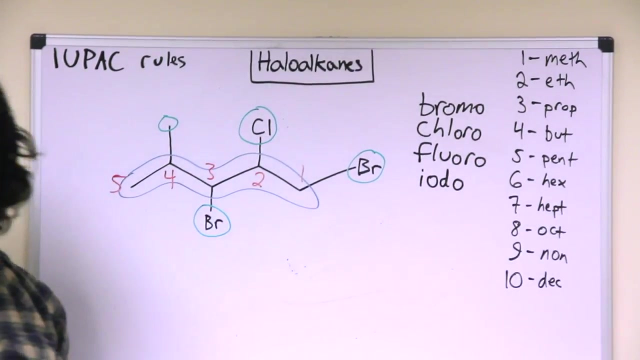 halogen groups, and these are going to be abbreviated thusly, we have bromo, chloro, fluoro and iodo, depending on whether it is a bromine, chlorine, fluorine or iodine atom, and the rules for alphabeticity are also. 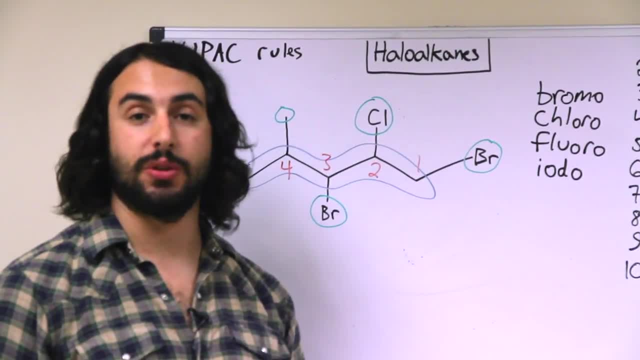 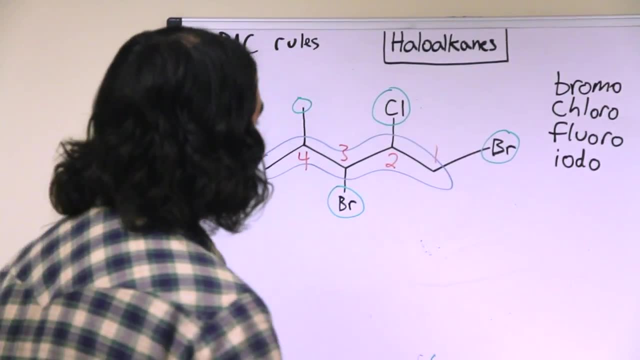 the same. so the substituent that occurs soonest alphabetically is bromine, and we have two of them, one on carbon 1 and another on carbon 3.. so we will list that first, but we do have two of them, so we will list them simultaneously. it's: 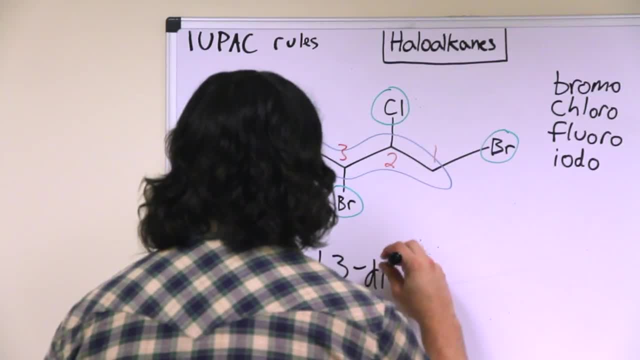 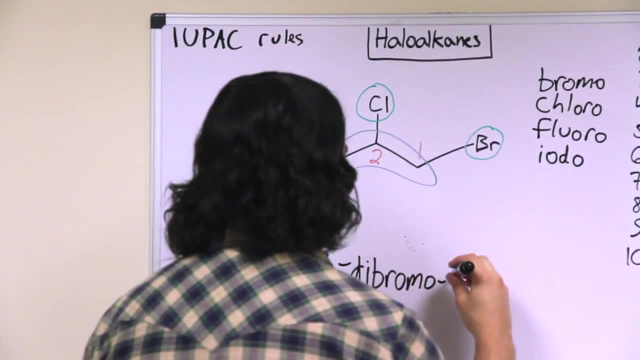 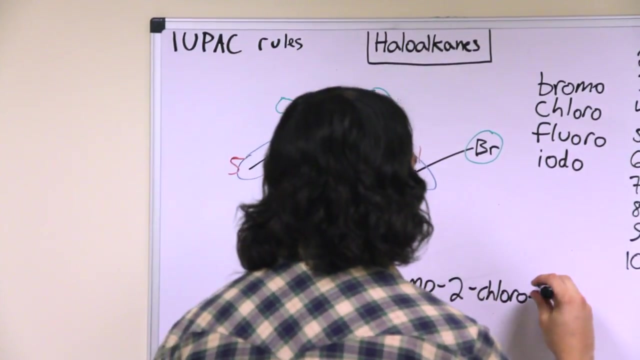 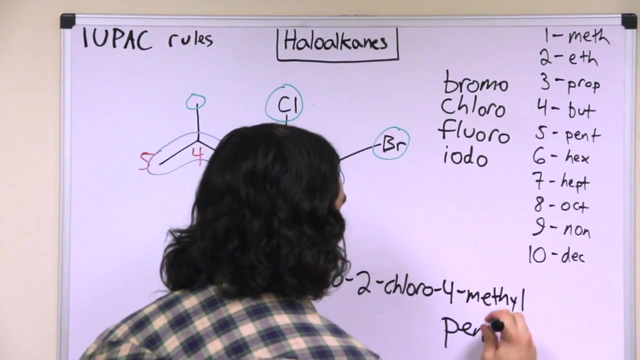 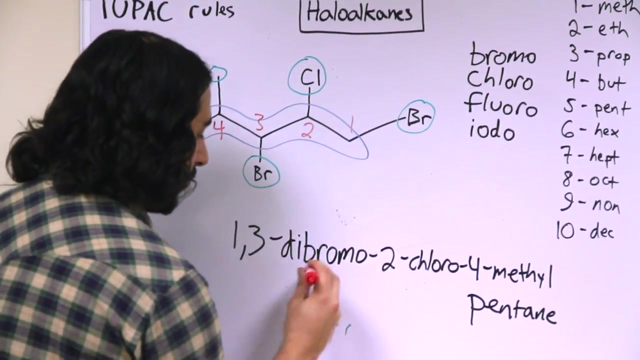 going to be 1,3-dibromo. next we have a chlorine on carbon 2, so that is 2-chloro, and then, lastly, the methyl group on carbon 4, and it is a pentane. so once again, alphabeticity dictates that we are going to have bromine before chlorine. 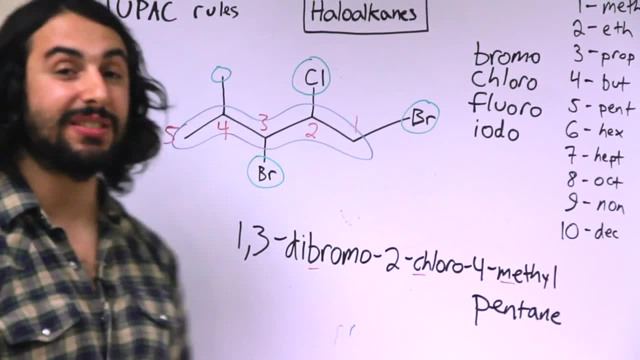 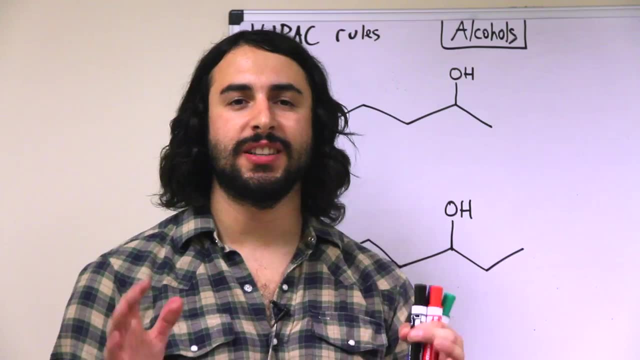 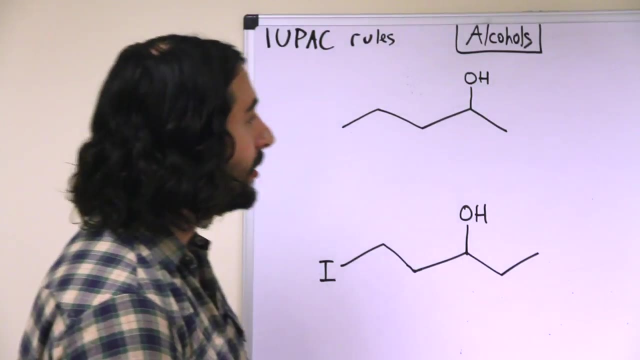 before methyl, and bear in mind that the prefix di- is not taken into account for alphabeticity. let's talk about another substituent, the hydroxyl group. a hydrocarbon that bears a hydroxyl group is called an alcohol, so a hydroxyl group is the OH group that we see. 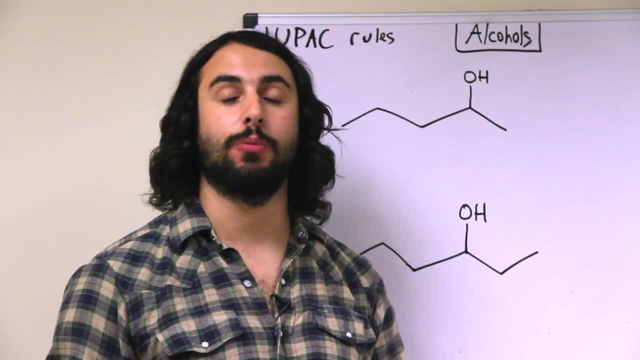 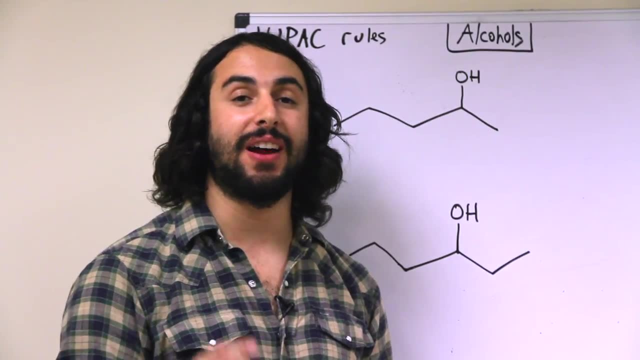 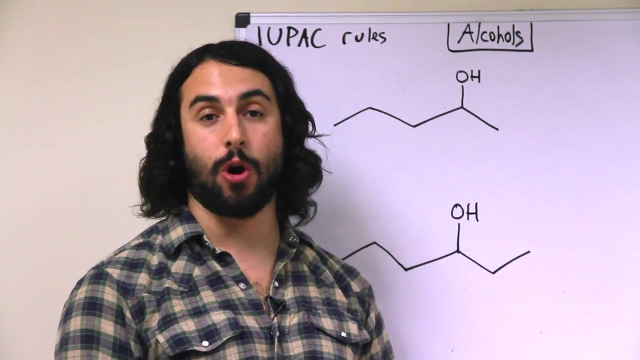 here. the hydroxyl group is a group that modifies the behavior of a molecule sufficiently that we deem it necessary to modify the suffix of the molecule. so this is no longer going to be an alkane, it is an alcohol, and so the suffix is no longer "-ane", it's "-ol". 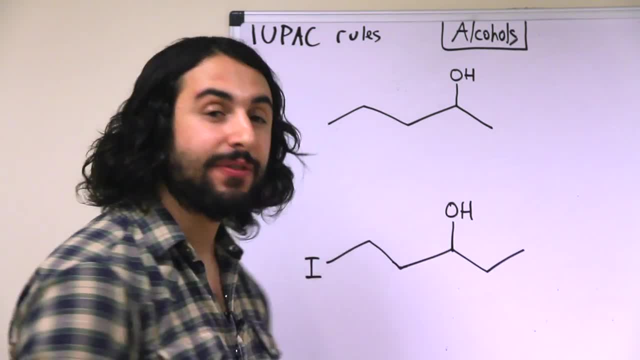 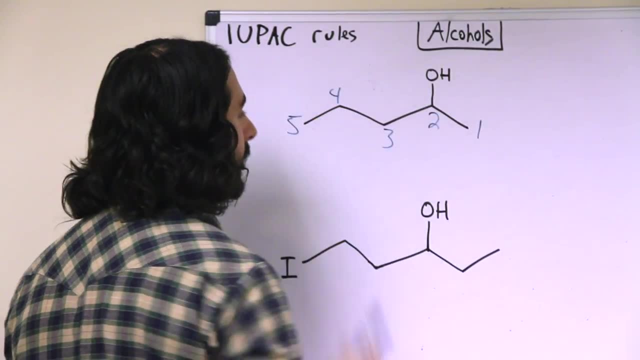 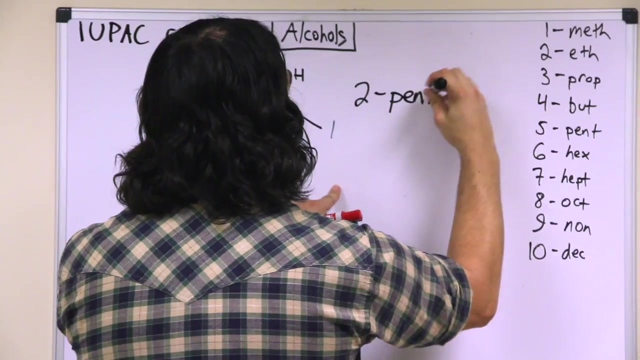 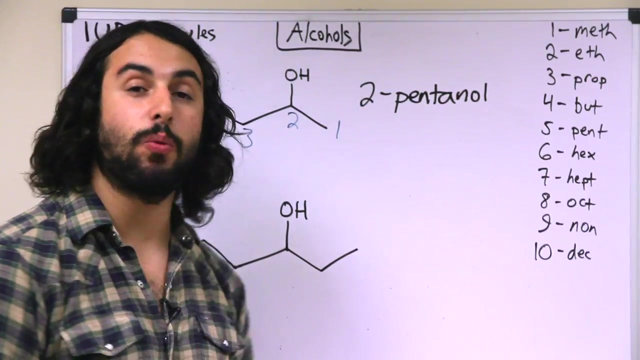 so here we see that we have a 5-carbon molecule. we're going to have to number this right to left to give the hydroxyl group occurring. so now what we are going to call this is 2-pentanol. so we are going to have to say where the hydroxyl group occurs. but we are going to list the. 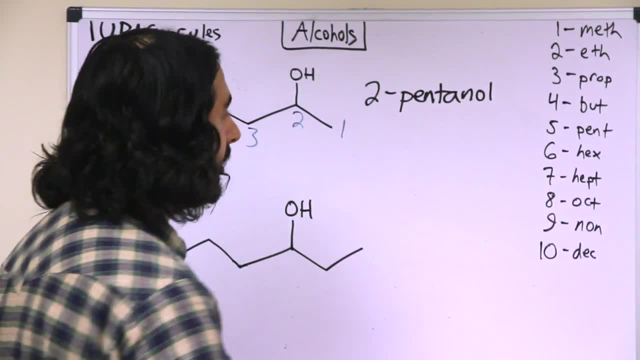 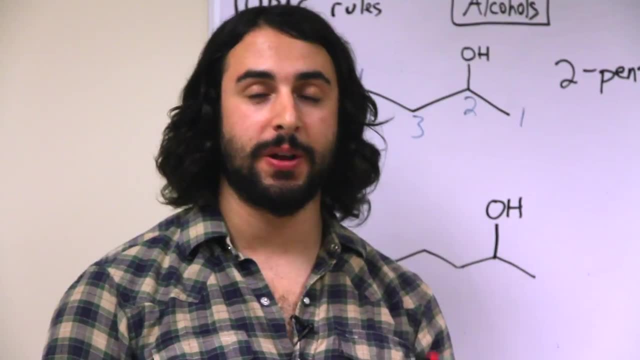 presence of the hydroxyl group in the suffix of the molecule now. so this is "-ol" for an alcohol. now, here's the thing: the hydroxyl group takes priority. it takes priority over alkyl and halogen in terms of the priority of numbering left to. 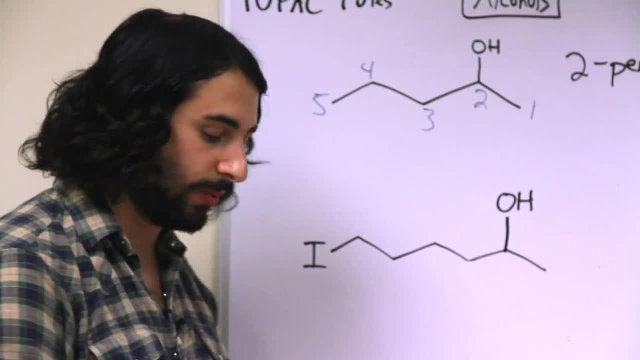 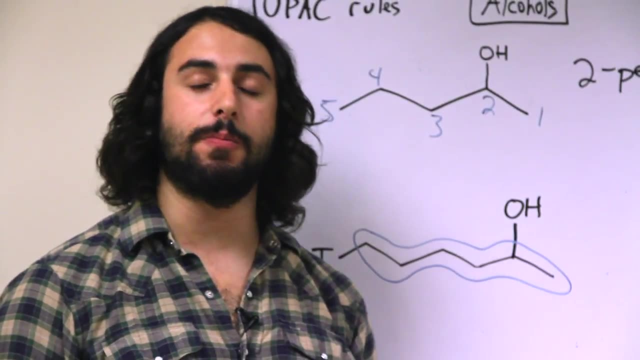 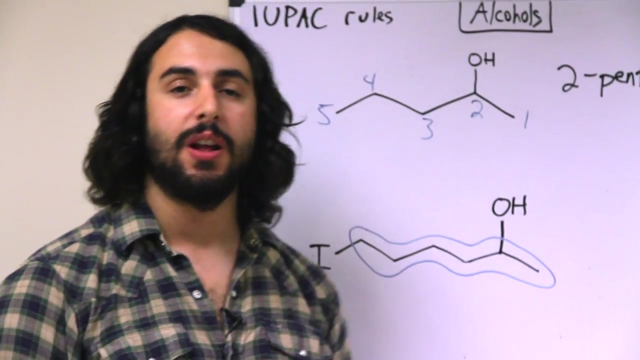 right or right to left. so what that means is, for this example, we will identify the longest carbon chain, just as we normally do. however, whereas before we would probably have decided to number left to right, because an iodo group would occur on carbon 1, if we number from the left, because 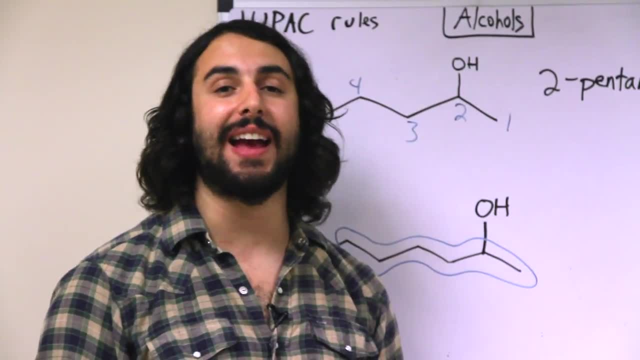 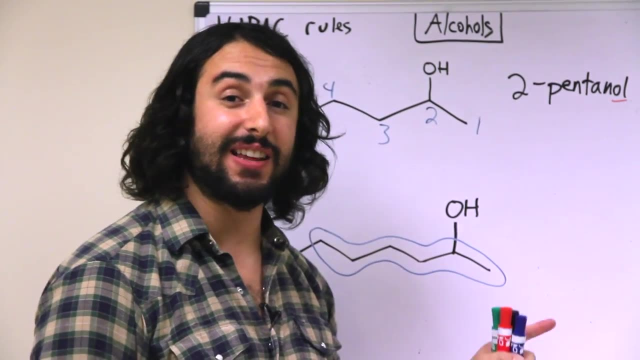 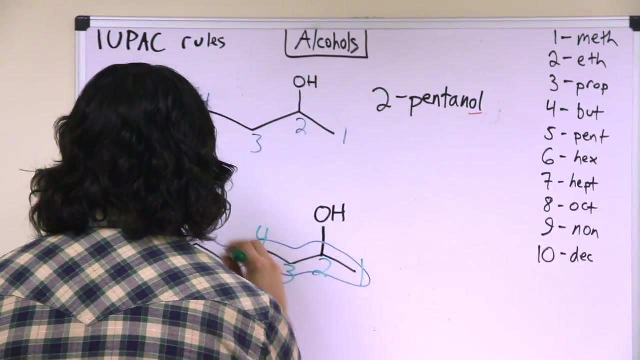 the hydroxyl group takes priority over any alkyl or halogen substituent. we are going to have to number from the right to the left because that will specifically give the hydroxyl group occurring soonest. so we will number this way only for the reason that it gives the hydroxyl group occurring. 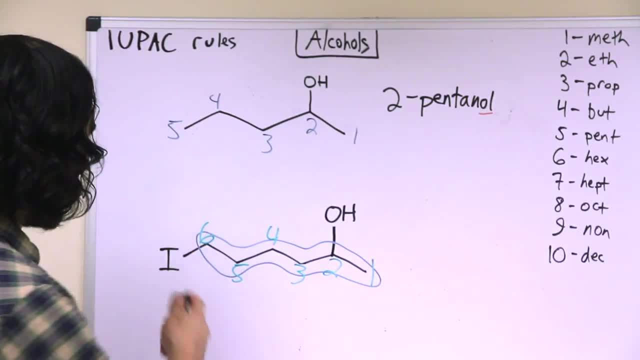 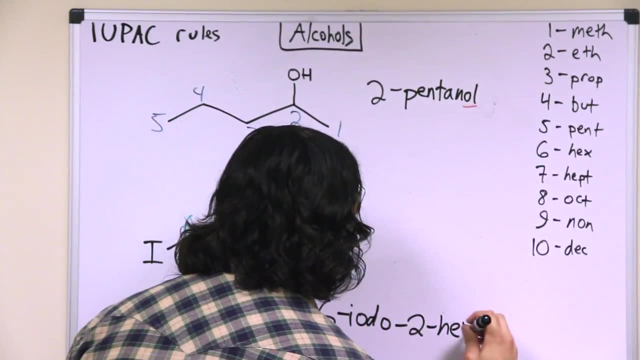 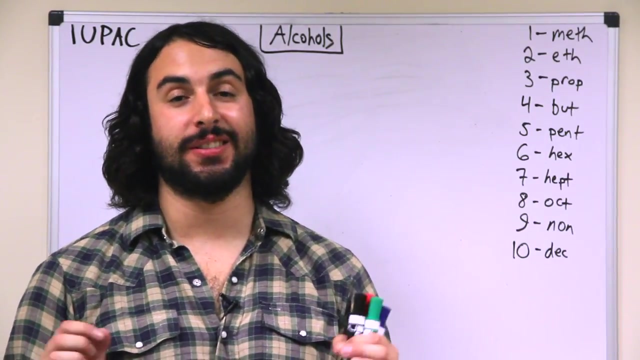 sooner. so now we will simply, as you would expect, list what we have. we have 6-iodo 2-hexanol. let's summarize what we've learned today: if we want to name a simple hydrocarbon, there are two things we must do. 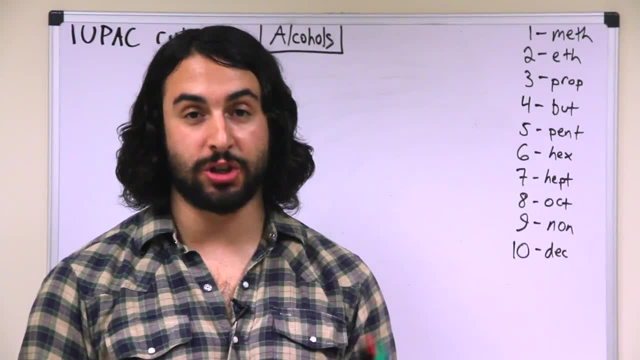 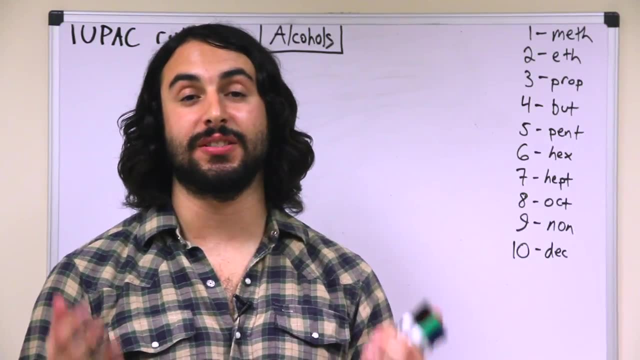 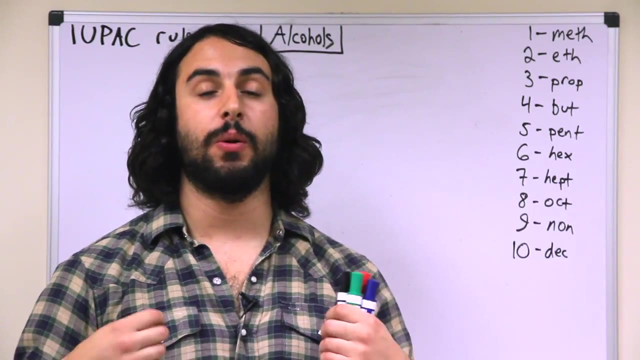 the first thing we have to do is identify the longest carbon chain. then we have to number that chain from left to right or right to left, depending on which direction gives a substituent occurring soonest. if a substituent occurs on the same carbon, regardless of which side we start from, we